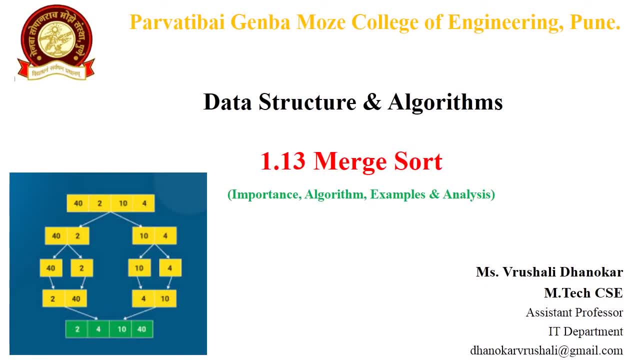 Good morning everyone. I am Rishali Dhanavkar, Assistant Professor, IT Department. In my last video, we learned about bubble sort, insertion sort and quick sort technique. Hope you have watched my previous video. Now, in this video, we will learn about merge sort technique. 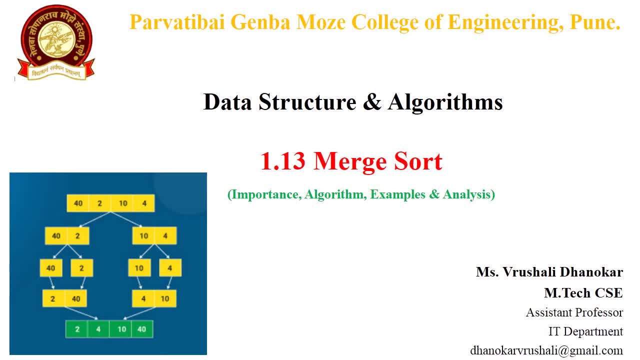 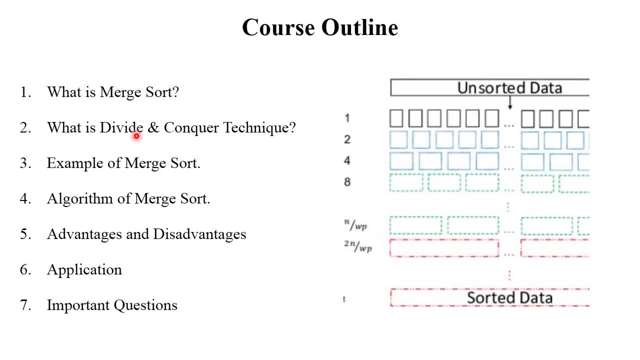 So let's see how exactly merge sort work Next. So following points are covered in this video, which includes what is merge sort, divide and conquer technique, examples, algorithm advantages and disadvantages, their applications and also some important questions which frequently. 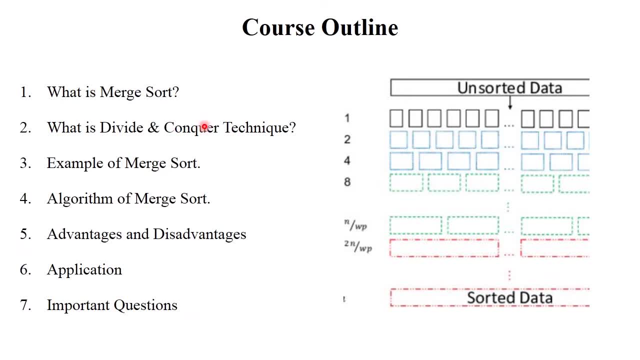 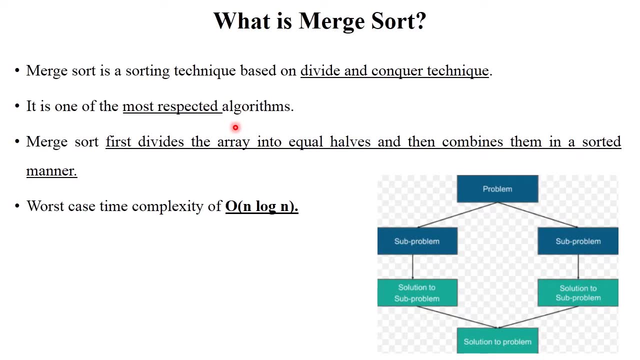 asked in SPPU exam pattern. So let's see one by one, what is merge sort Next? So merge sort, Merge sort- is one of the finest sorting technique and this technique is based on divide and conquer approach. In my previous video I already explained quick sort technique. Quick sort also used 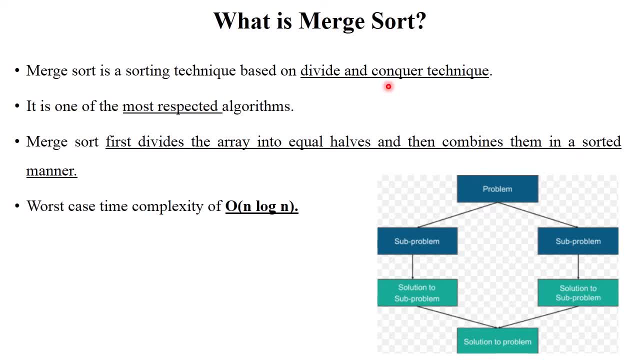 divide and conquer approach and merge sort also used divide and conquer technique. It is one of the most respected algorithm And the concept of merge sort is first divide the array into the two equal half and then combine them in a sorted manner, Clear And 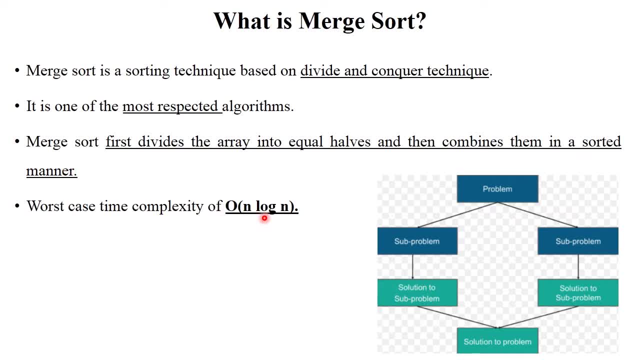 the worst case time, complexity of merge sort is big O and log N. You have to just remember that the order where you divide and conquer the array is based on the order from which you divide and conquer. Okay, So this is the concept of merge sort Problem can be divided. 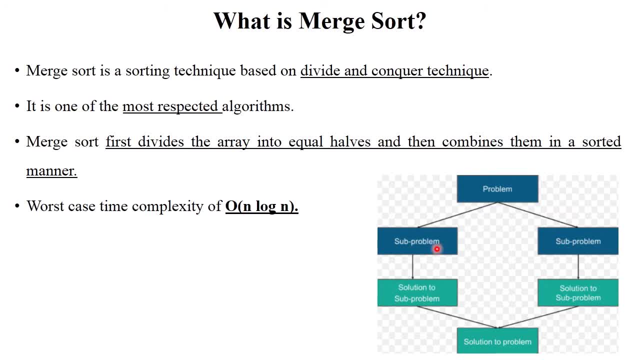 into the two equal half. ie subproblem against subproblem again is divided into the two half. Find out the solution means arrange in sequential order And after that the sequential data or sorted data combine in final result: Clear: This is the concept of merge sort Next Before. 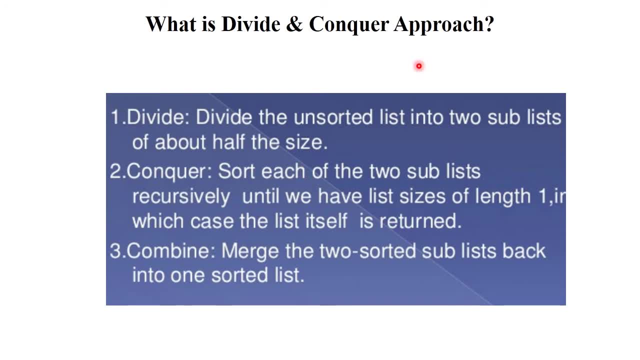 starting example. first, what is mean by divide and conquer approach i already explained in my previous video. here we will just take a review of divide, conquer and combine approach. what is mean by divide? divide means unsorted list, divided into the two equal half part. this is called as 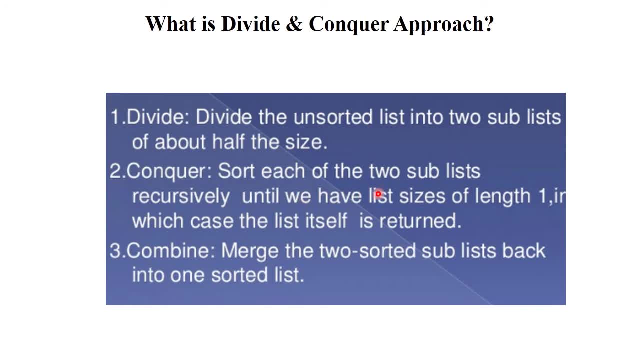 divide, conquer. conquer means sort each of the two sub list recursively until we have a list size of length, one and last. combine. combine means merge the two sorted sub list back into the one sorted sub list. clear. this is called as divide, conquer and combine approach. divide means divide, partition. 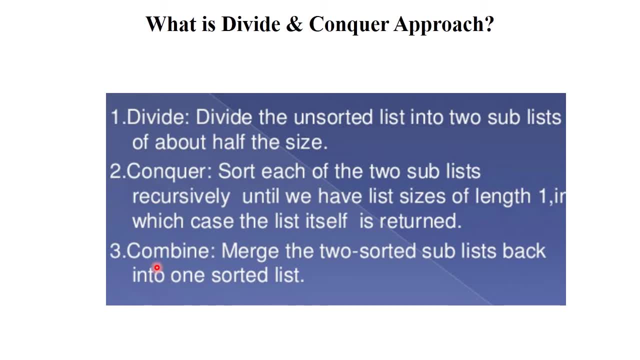 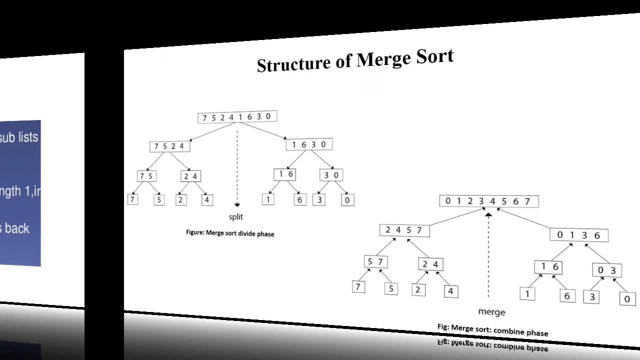 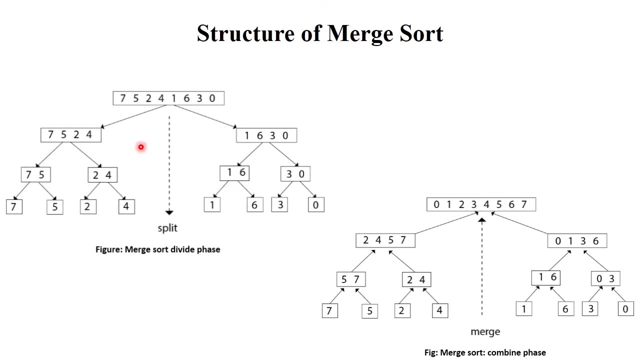 conquer means sort those divided data and combine means after sorting, combining into the one sorted list. clear next. so here structure of merge sort, or we can say it's one of the example of merge sort. see here there are two: technique split and merge split. use technique top to bottom approach and merge bottom to top approach- clear. so see first divide phase. okay. 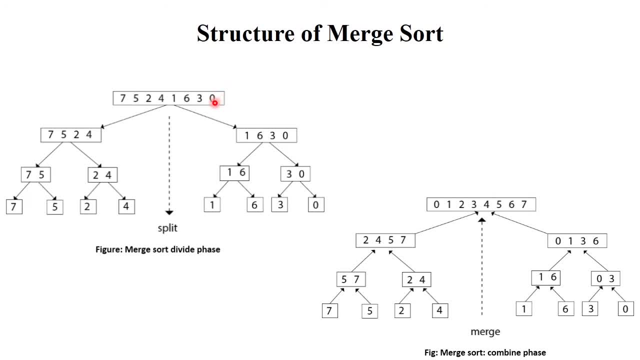 so the given input is seven to zero, means there are total eight numbers. okay, so it can be divided into the four and four equal parts, that is, seven to four and one to three. clear again is divided into these two elements like one, six and three, zero. clear and again is divided into the single. 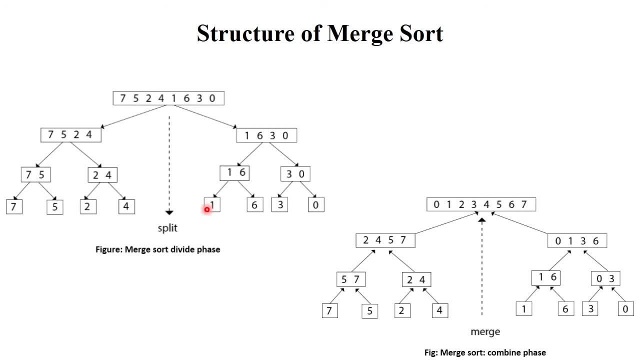 element. so you have to divide the unsorted data up to the single elements: clear. this is the hierarchical structure of merge sort. okay, this is the first step. that is, divide phase or split phase- clear. so after completion of first phase of divide division, you have to move here merge phase or. 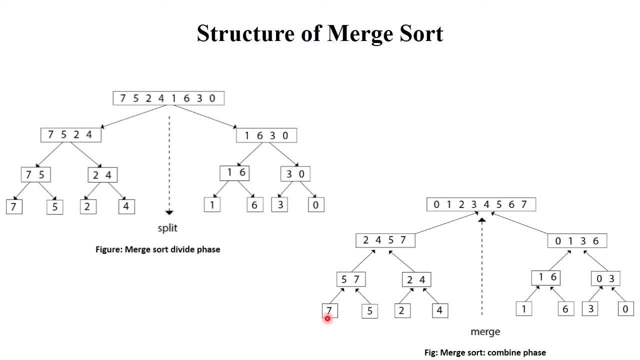 combined phase. okay, so after sorted the you have to use merge all together and can consider it is weird because of it. here merged is not step will be divided. so after sorted the device is, will normality have to combine data from left to right side? okay, so 7 and 5. these are the sorted division phase. 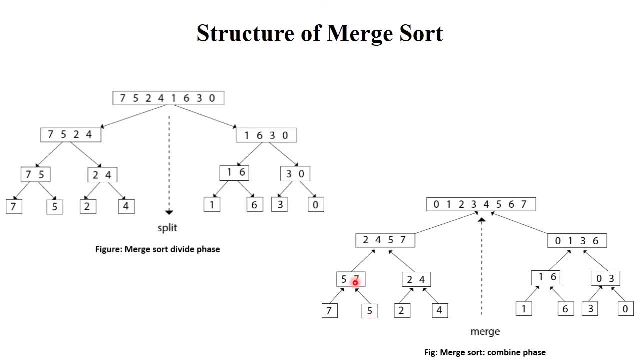 element, okay, you have to combine or merge it. so while merging or at the time of merging, you have to do in sorted format like 7 and 5 and after combining it's 5 and 7 in sorted manner. clear, 2, 4 combine into the one part, 2 and 4. as it is. again, these two element combine into this format. 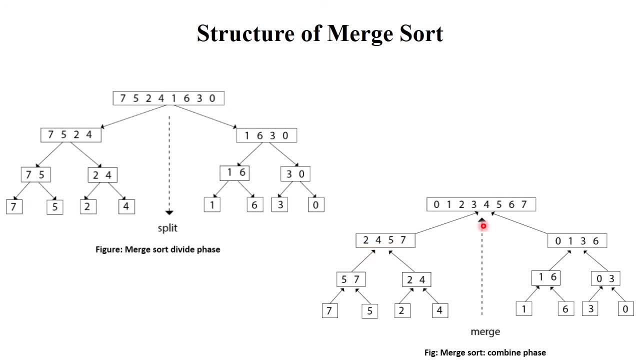 2, 4, 5 and 7 in sorted format: okay, similar to right side. okay, and at last, 2, 4, 5, 7, this part and this part, combine it into the one single element or single sorted list, that is 0 to 7. 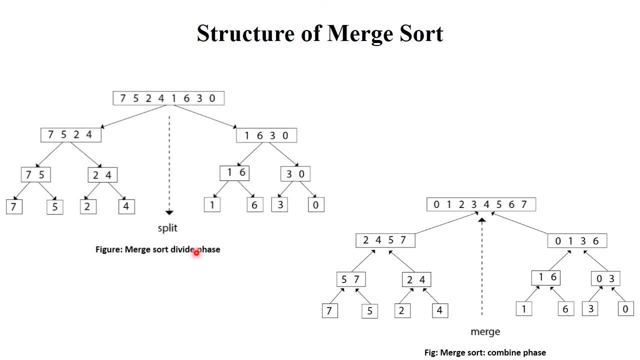 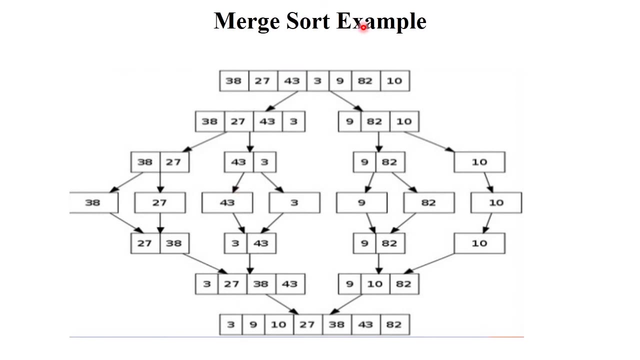 clear. so this is the structure of merge sort: first phase split, second phase merge split work top to down and merge work bottom to bottom to top, while sorting clear next. this is again the example of merge sort. now see here: the given input is 38 to 10 means there are 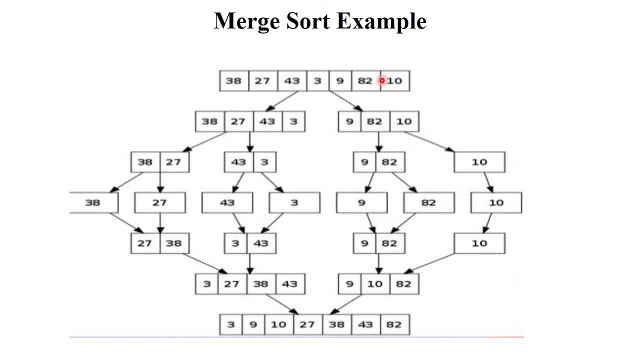 total: 1, 2, 3, 4, 5, 6, 7, 7 elements. okay, so how to sort it? you have to combine either. it is you have to sort is either 3 or 4 or 4, 4 or 3, okay, so 4 plus 3 means 7. okay, again this element sorted into the 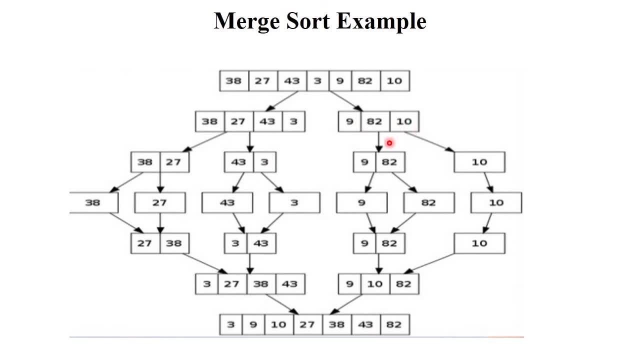 2 and 2 equal half parts. okay, again, is sorted into the 2 and 2 equal half parts. okay, so this is 2 and 1 part. okay. again is sorted or divided into the single element up to the single element, so this is called first phase up to the single element. like 38, 27, 43, all are in separate. 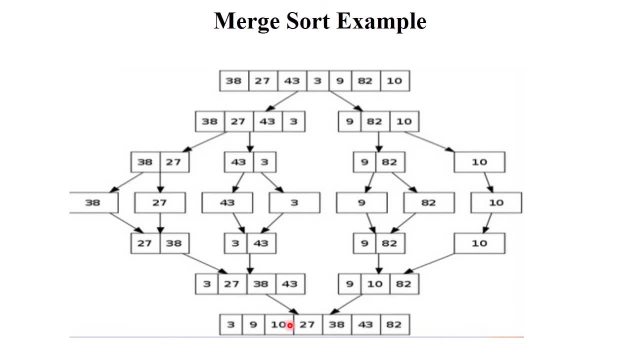 elements: okay, and after dividing phase you have to use merge phase or combined phase. so 38 and 27. after combining it becomes 27 and 38 in sequential or sorted format. okay for 43 and 3. so after a combining it becomes 3 and 43. okay, again, you have to use combine on this 9 and. 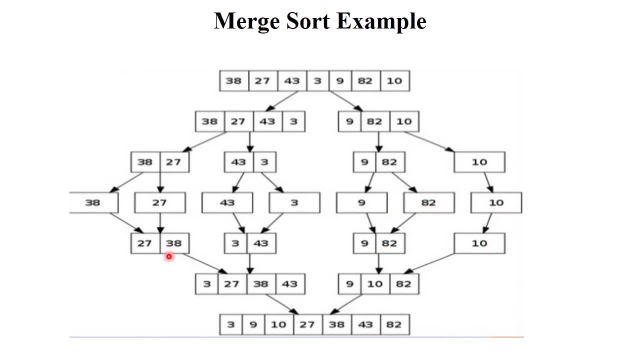 82 and 10. as it is clear again, you have to merge 27, 38, 3 and 43 into the one combined phase. okay, that in sorted format, 3, 27, 38, 43, etc. okay, and at last you have to combine remaining two. 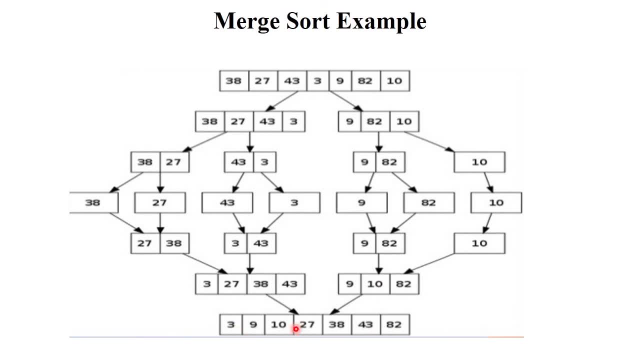 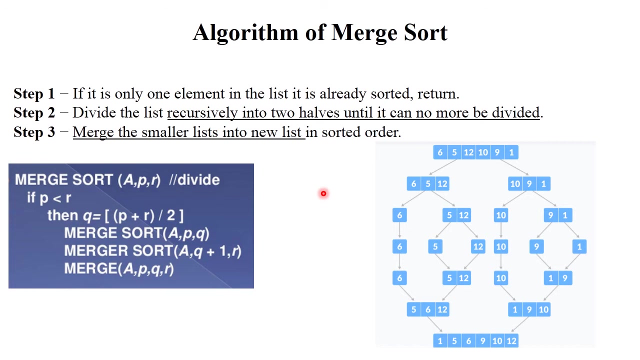 list in sorted format: 3, 9, 10, 27, 38, 43, etc. clear. so this is called divide and this is called combine phase: this is unsorted list and after applying merge sort it becomes sorted list. clear next. so algorithm of merge sort: i already explained here examples of merge sort, so step: 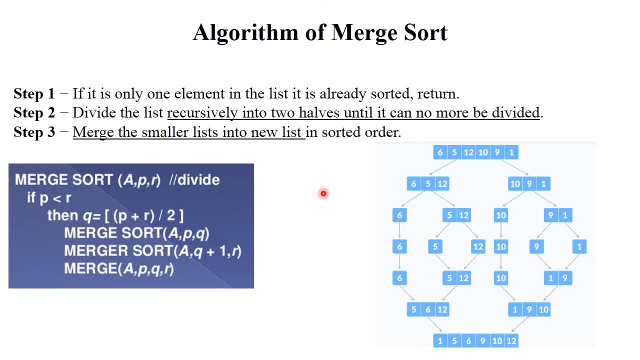 wise solving pattern of examples, which is also called as algorithm. algorithm of merge. sort means step by step sequence. okay, so step 1: if in the list there is only one element, then list is already sorted right. second step: divide a list recursively into the two half part until it can more be divided. recursively means this list can be divided into the two. 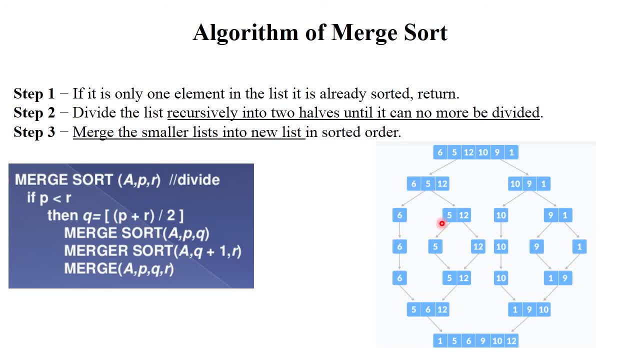 equal parts. again this list can be divided into the two equal parts. and again this list can be divided into the equal parts until there can be no more division approach. okay, so this is called recursive right and merge. last step is merge the smaller list into the new list in sorted order, and after division you have to combine in. 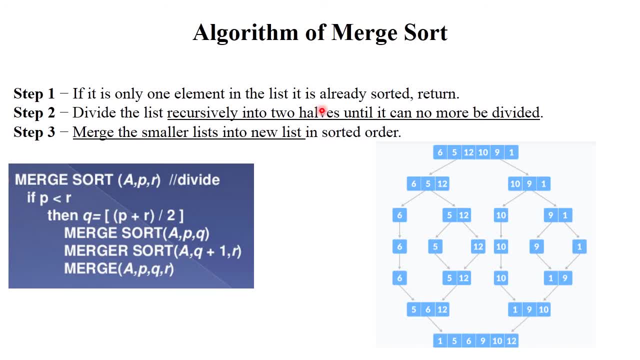 sorted format clear. so this is called as algorithm of merge sort here inいる програмmatic approach. like merge sort array. p means division. like p and r first to last element. okay, if p is rする t power chainsidersor, merge sort. first you have to divide into the two part, p plus r divided by two. 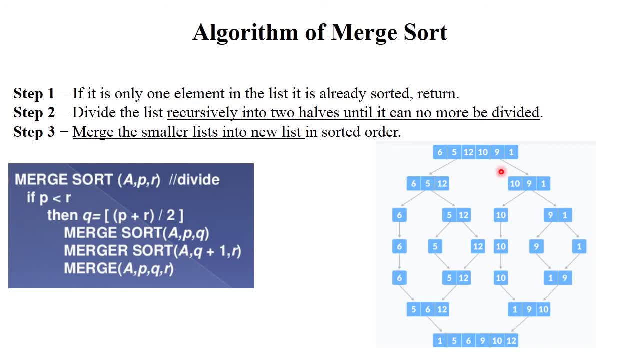 means this list can be divided into the two half part. okay, again you have to apply merge sort. again you have to apply merge sort on this list from p to q and q plus 1 to r. clear. and at last you have to apply merge operation. okay, merge. 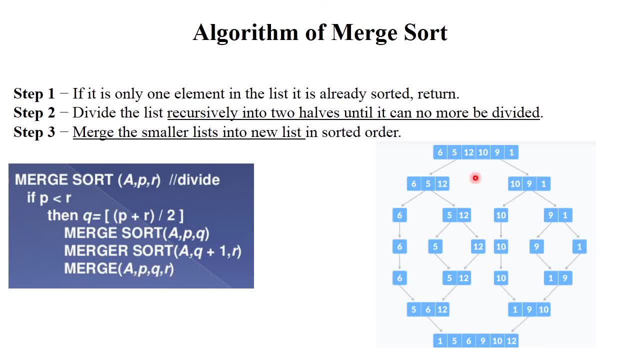 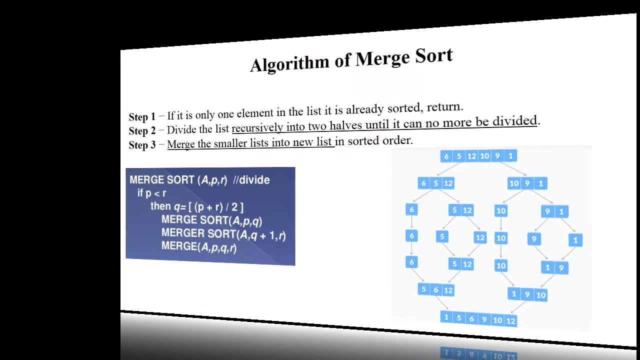 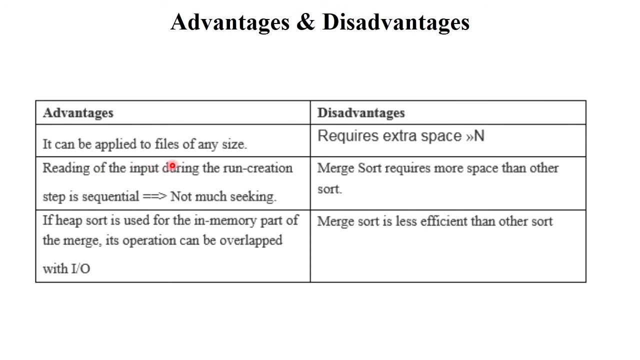 means p, q and r, all list you have to combine with each other in single array, clear. so this is the step of merge sort. next, advantages and disadvantages of merge sort. the main advantages is it can be applied to file of any size. you have to use anywhere reading the input during the run. creation means sequentially you. 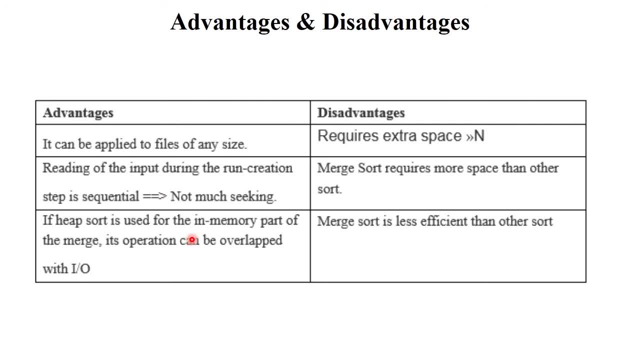 have to solve each and everything. if heap sort is used in main memory part, the merge operation can be overlapped with input output. heap sort is another part. okay means all the disadvantages of merge sort are the same. merge sort is overcome in our next. that is heap sort. okay, but the disadvantages is it. 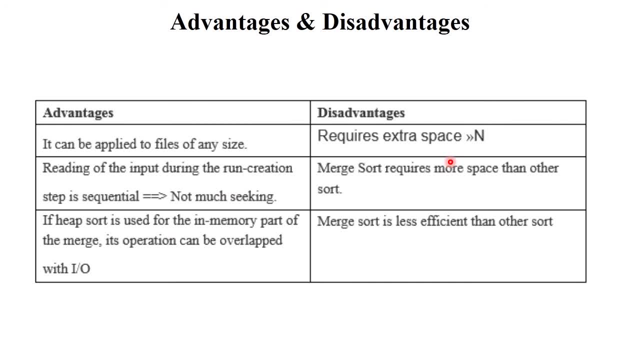 requires extra extra space. okay, if there is large number of list. so for division purpose, sometimes it used extra space. merge sort requires more space than any other sort. okay, so space complexity issue in merge sort. merge sort is less efficient than any other sort. okay, so as per the requirements we have to use each. 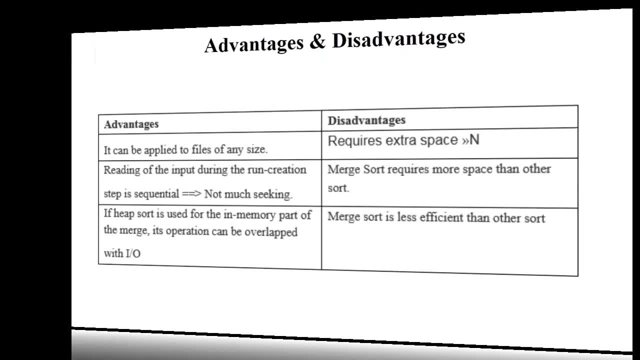 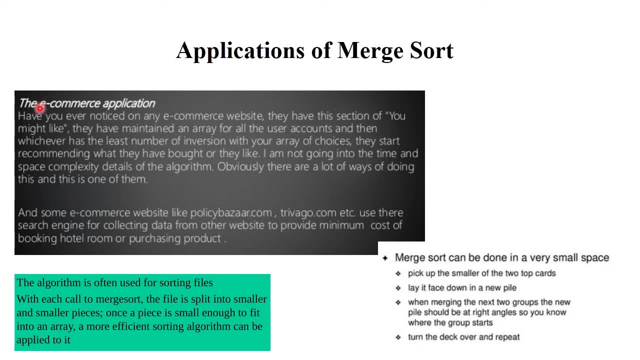 and every technique. okay, next here are some applications of merge sort where merge sort are used in real life. the first ecommerce application: have you ever noticed an ecommerce website? they have. this section you might like means all the like elements are stored into the one list or bucket, right, so it maintain the array of the user accounts and whichever. 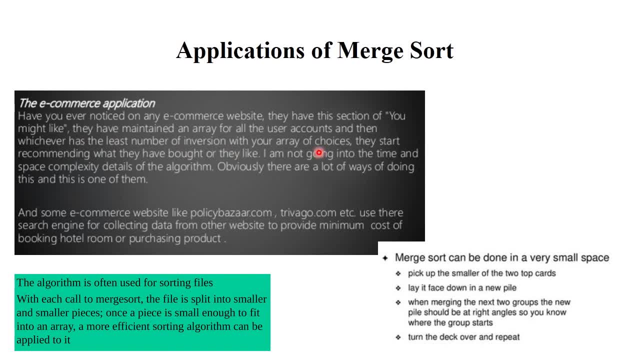 the list number of inversion with your array of choice means according the choice you have to sort it. the Each and every list. okay. Some e-commerce website like policybazaarcom, trivagocom. they use a search engine for collecting data from other website. 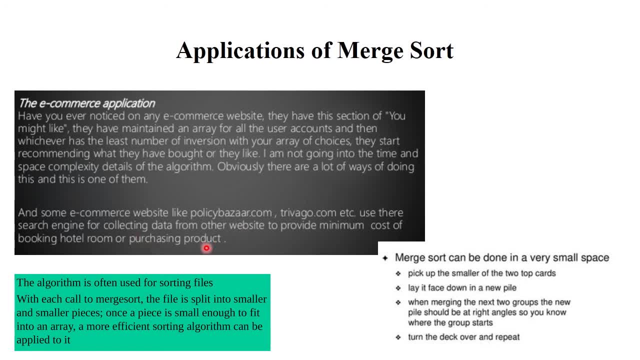 and provide minimum cost of booking hotel room, purchasing product, etc. Clear, At that time Merge Sort technique is used, Means they search and divide each and every price of that particular product And at last they combine those product into the one list. okay, 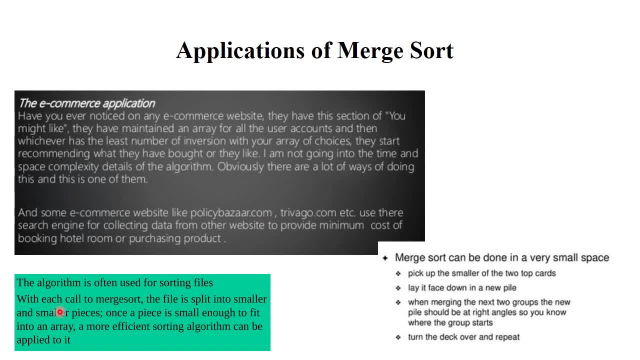 The algorithm is often used in sorting files. With each call to Merge, Sort, the file is split into the smaller and smaller piece. One piece is small enough to fit into the array Again. it's more efficient. sorting algorithm is used. Clear. 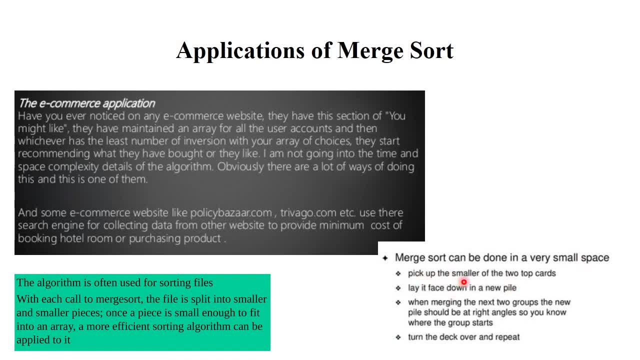 Merge Sort can also done in very small space. It pick up the smaller of two top cards, face down into the new pile again merge the two groups into it, okay. So this is an example of applications of Merge Sort Clear. 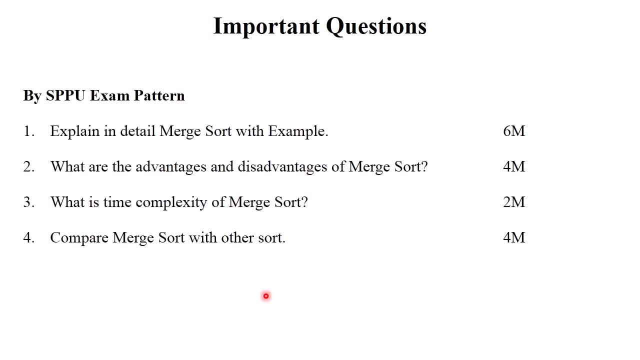 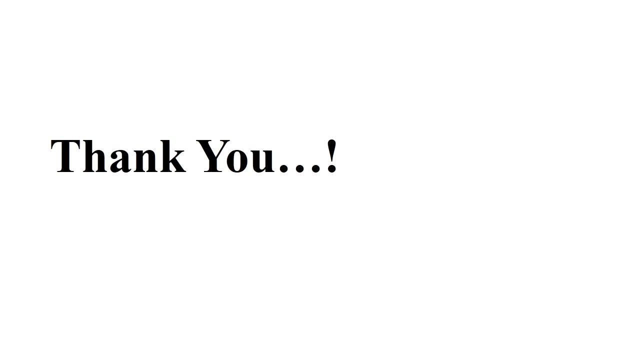 Next. These are the some important questions which frequently asked in SPPO exam: pattern, Explanation, advantage, disadvantages, time, complexity and comparison according to their marks. Okay, Next, Hope. so you understood each and every concept of sorting technique, or especially Merge Sort.